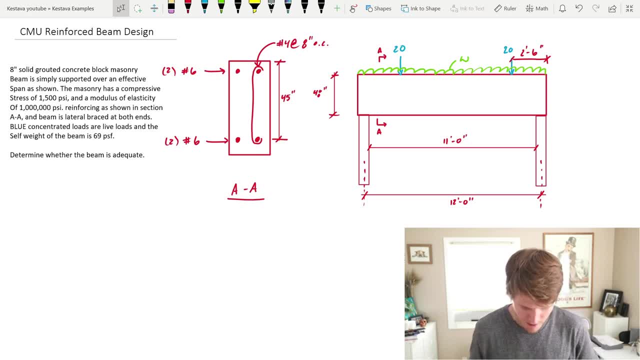 We have a simply supported beam that you can see there- Simple elevation view. I have the self-weight of the beam denoted in green that we need to calculate. And then we have two point loads that are two and a half feet from the edge of the beam That's actually going to be down to. 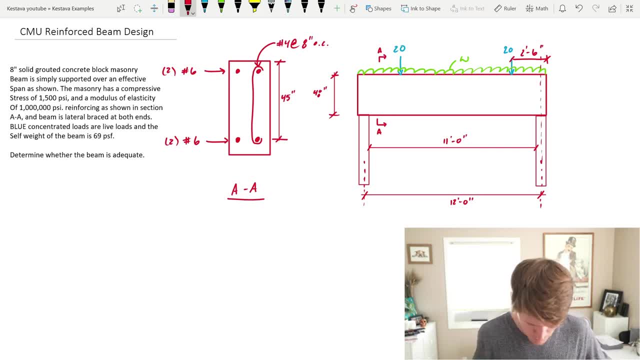 the center line of the support And that's the same on both sides, And you have a little AA cross section right there showing all the rebar in it And basically we have our design CMU properties over to the left, And then we have the center line of the beam And then we have the 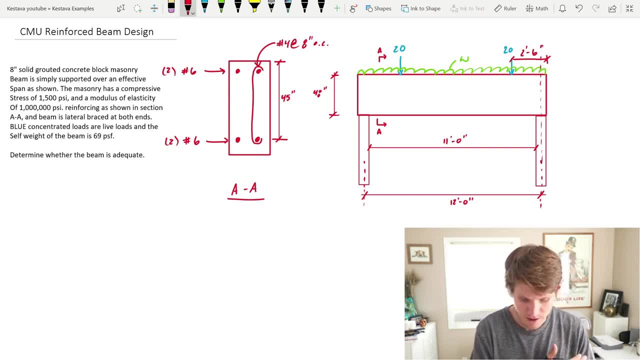 center line of the beam. And then we have the center line of the beam, And then we have the center left And we just need to determine: hey, is this beam adequate under the loading provided? So let's figure that out. Well, first of all, let's determine- We'll go green- What W is the? 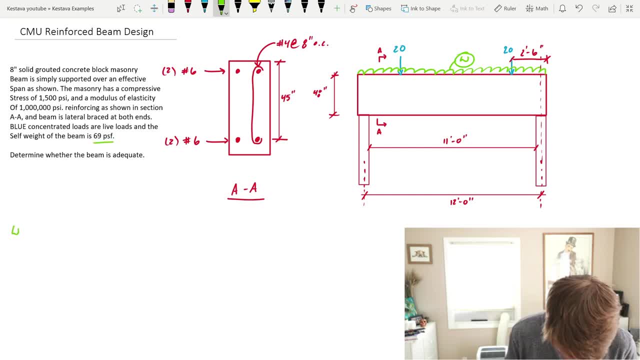 self-weight of the beam. Well, we see right here: 69 PSF for the self-weight of the beam Beam's 48 inches deep W is going to equal 276 PLF. We today. I'm going to switch back to red. 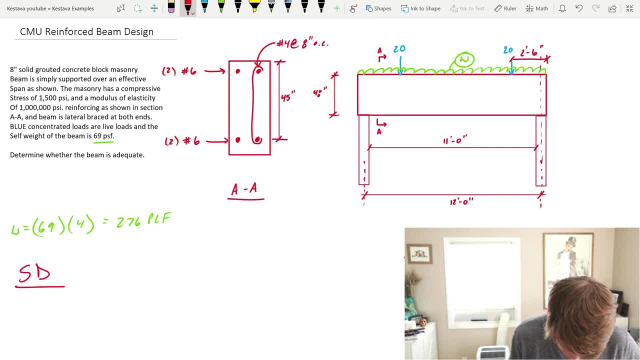 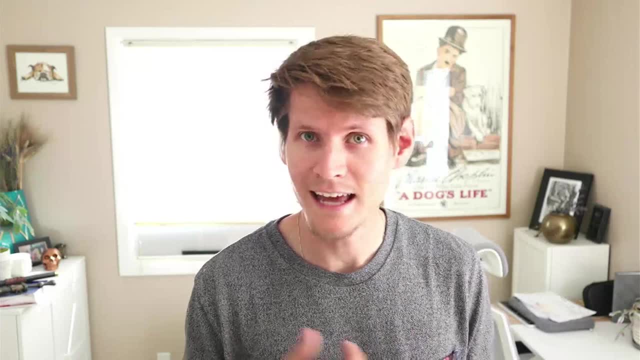 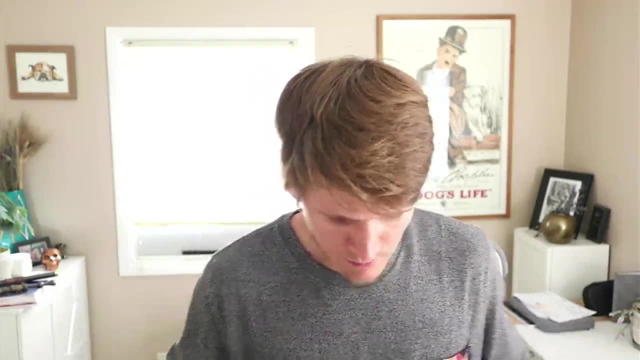 are going to be designing this whole thing per strength design- SD. So in masonry design you have two paths forward. You can either do allowable stress design- ASD- or you can do strength design or which that's in tandem with, like LRFD. So strength design you are going. 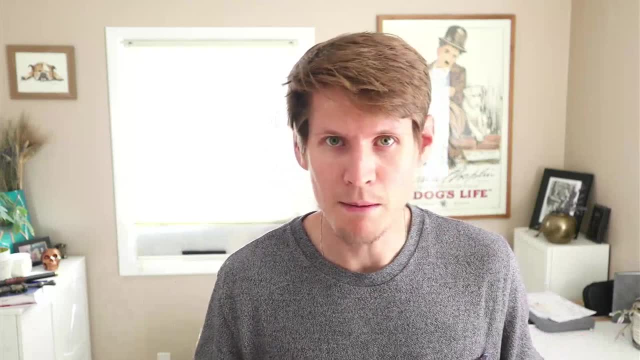 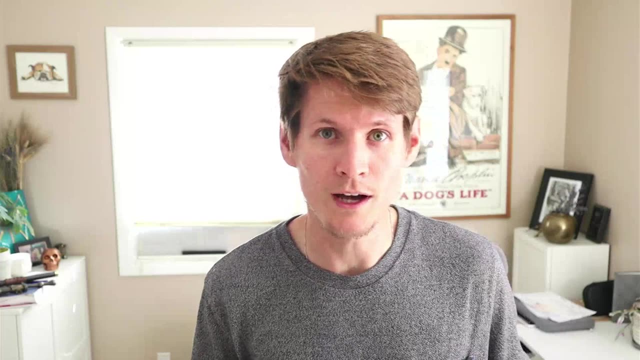 through procedures and using equations to determine if the member, the column, the whatever, has adequate strength to resist the total load on that member. Whereas for ASD, slightly different equations and you're determining if the strength of the beam is adequate or not. So you're. 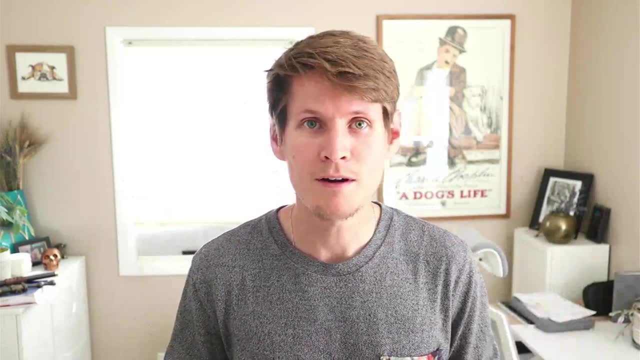 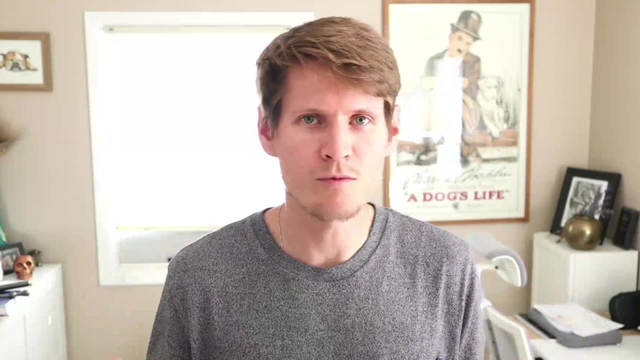 going to be doing strength design, ASD or which that's in tandem with like LRFD. So the stresses induced by the forces on the member are less than the allowable. stresses from the material properties that you're designing with Two different systems should get you relatively. 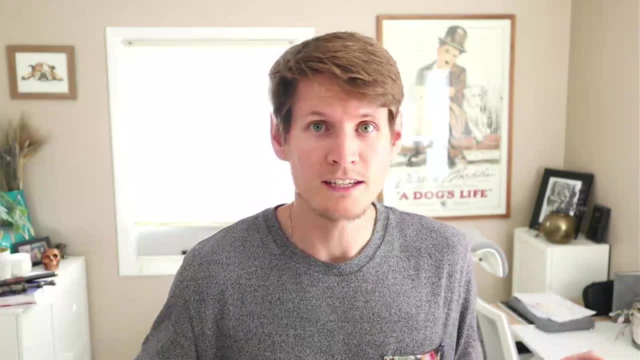 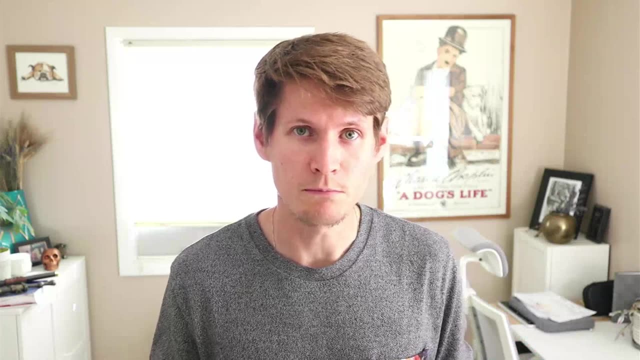 the same thing. Concrete, we all know that we need to do LRFD Strength design. Wood, you can switch between both. Steel, you can switch between both. CMU, you can also switch between both. But today, long story short, we're doing strength design. First thing we're going to do is get our 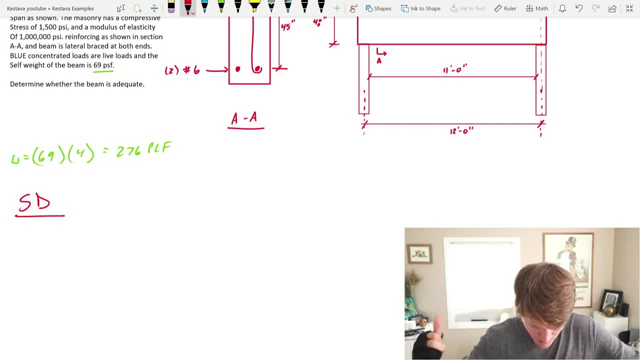 moments and I'm going to split them up between the moment-induced stress and the force-induced by the self-weight and the moment-induced by the live loads. MU dead load is equal to WL squared over eight. That gets us 4.97 feet. And then MU live load. I pulled the equation from the AISC. 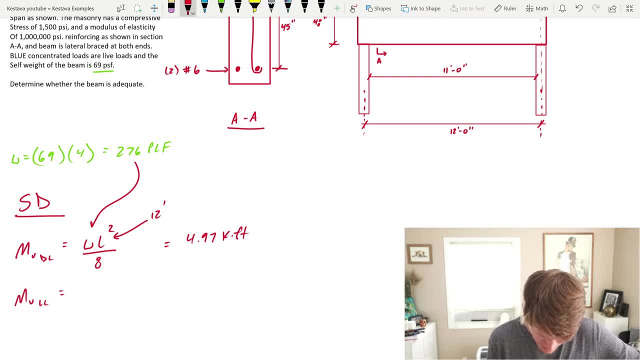 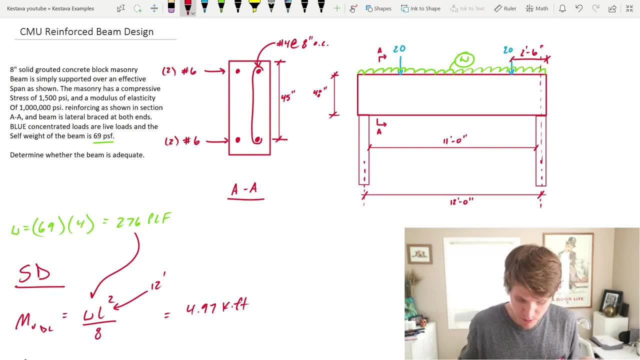 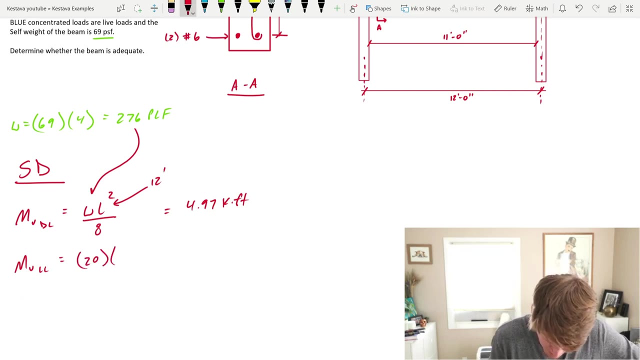 steel manual in the kind of the load tables that they provide there, where you have a point load to symmetric point load, symmetrically placed on a simply supported beam. That's what we have. So that gets you a live load of just 20, or your P times the distance to your simple support, which is 2.5 feet, And then 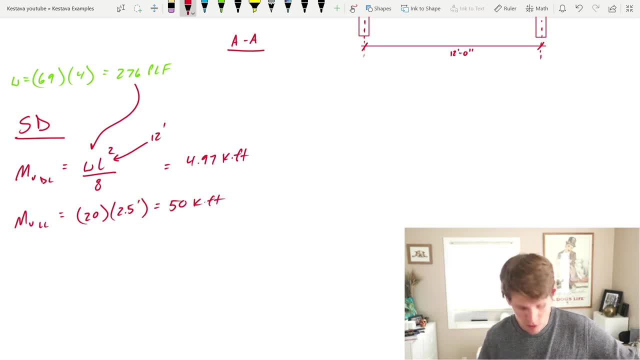 since we're doing strength design, we know that we need to factor our loads And for masonry it's 1.2 dead load plus 1.6 live load. That spits out. we'll call it. it's a beautiful summation. 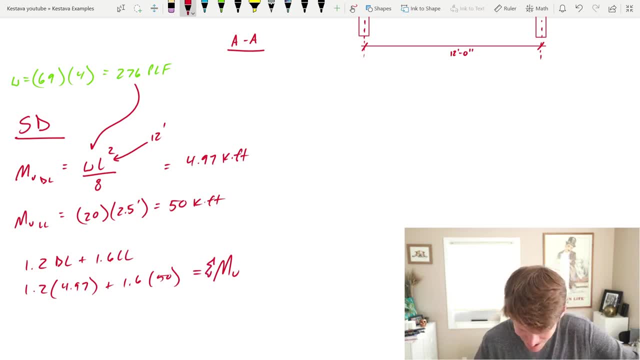 a summation, oh my god, a summation of moment ultimate equal to: we're going to round off 86 kip feet. There's that, And then we're going to round off. we're going to round off 86 kip feet. 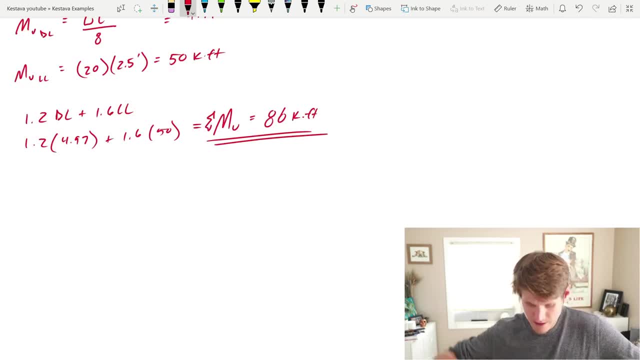 There's that, And then we're going to round off. we're going to round off 86 kip feet. There's that, Our demand, right there. Next, for strength design: you now need to find your A, Just like in concrete. 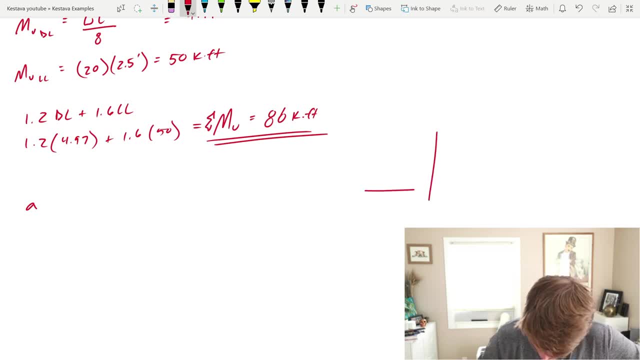 when you have your cross section and you have your steel down below here and then you have your compressive zone up above, denoted some A, your FYAS for your tension, and then your compression and all of that jazz and you have your stress. stress and your strain. 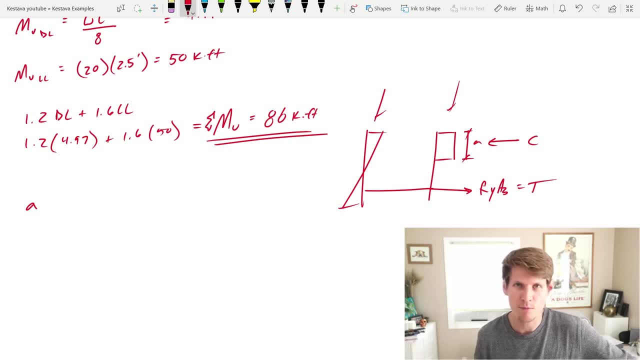 same exact thing, just slightly different variables for your properties, because CMU is just slightly different than concrete, but it is the same background. So A is equal to ASFY over 0.8, so there's one change there: B times F, prime M, So concrete. for all of you who may be jumping in, 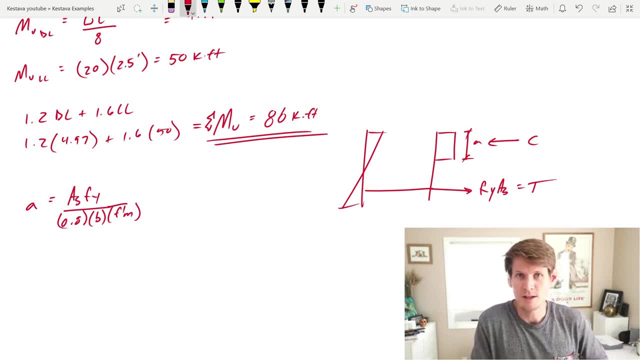 here for your first time. you have F prime C, that's the compressive strength of the concrete. F prime C, C for concrete. We have F prime M- M for masonry. That's really the big difference there. And then we don't get that 0.85,, we get 0.8, so slightly different. So we're going to round off. 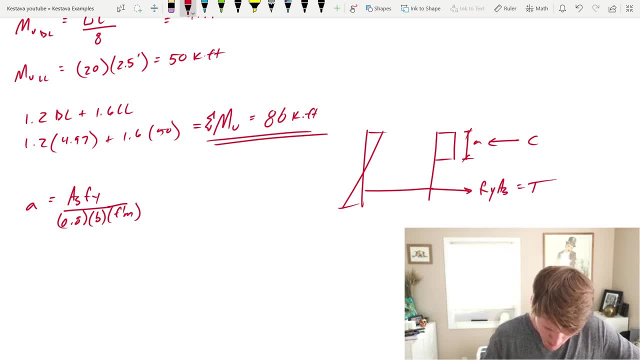 slightly less there, but everything else is the same And we know from up above that we have all the variables that we need, AS we have two number sixes. so we're just looking at the bottom- if I come over here- only the bottom- reinforcing steel. I know we have some up top in the compressive zone. 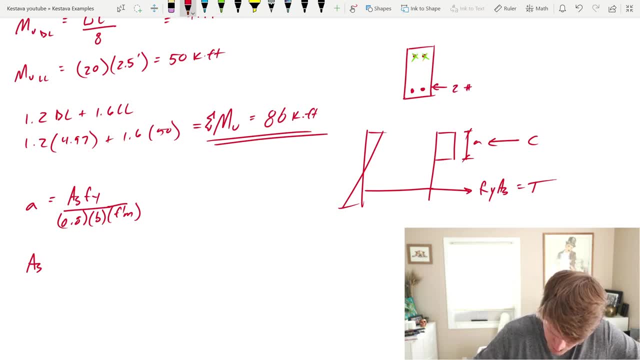 but we're going to ignore that. As it was up above, it was two number sixes. I got my Chrissy student detailing sheet. still use this thing to this day. Look down two number sixes or one number six. 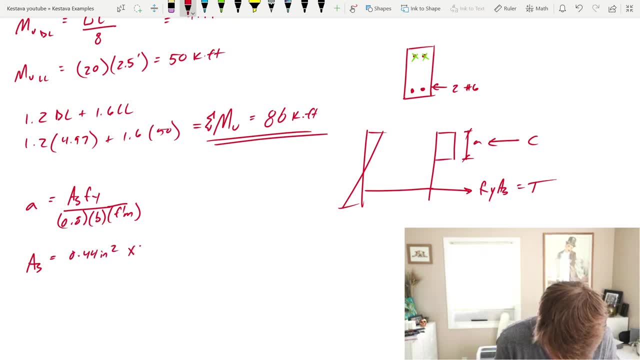 is 0.44 inches square. We have two of them, so AS is 0.88.. This is regular rebar, so 60 KSI steel B. it said above that we have eight inch masonry block, but you need to kind of pump the brakes there, Masonry. 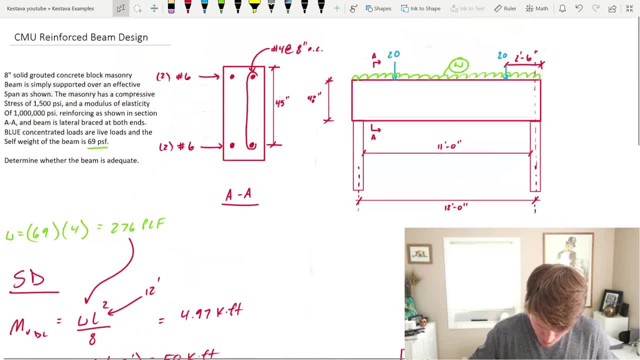 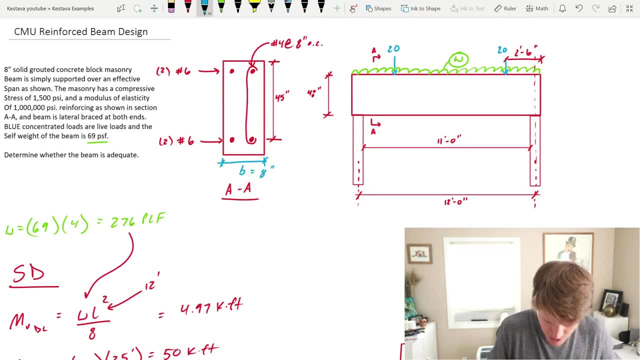 again is a little funky, So I'm going to scroll up to the top here. I'll go blue, although you might think, well, this is B, let's start there. You might think, oh, eight inches, boom, let's. 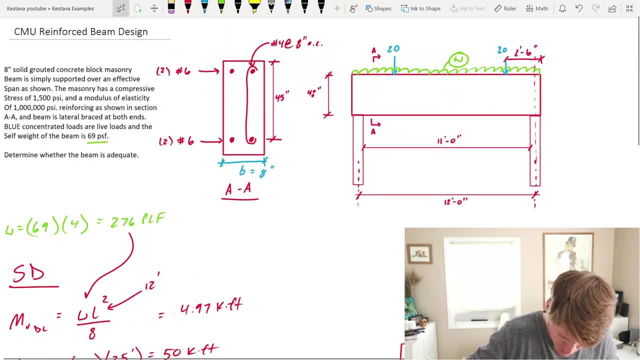 move on. Unfortunately not quite, as I'm jumping all over the place. It's actually seven and five eighths inches for an eight inch block, So it's just kind of like wood a little bit, where you have like a two by four, but that's actually one and a half by three and a half inches- Masonry, same. 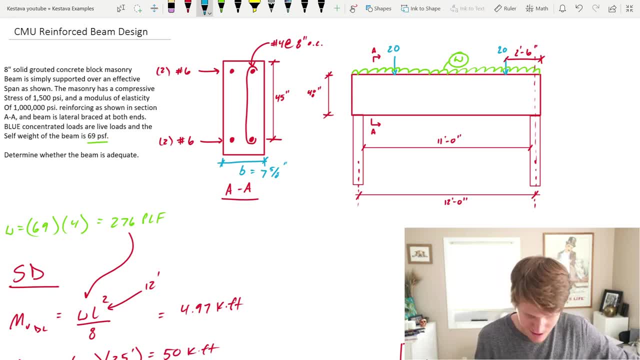 thing. You have six, four inch, six inch, eight inch, I think. you have 10 inch, 12 inch, but they're not exactly those dimensions And you're going to want to take the slimmed down dimension because you can't account for that little itty bitty extra. You want to make sure you're using. 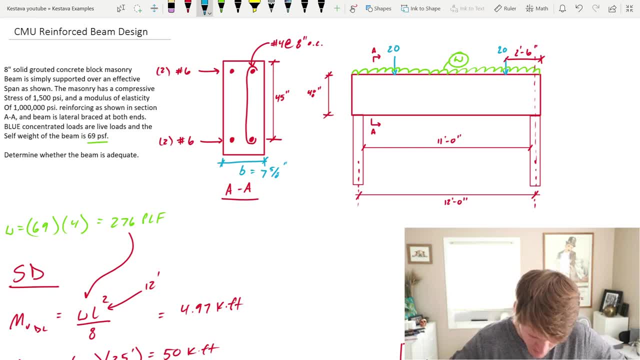 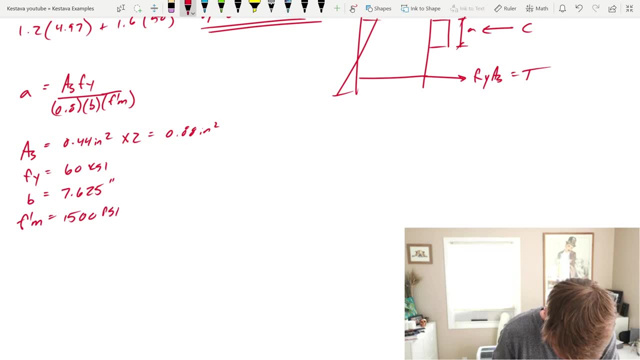 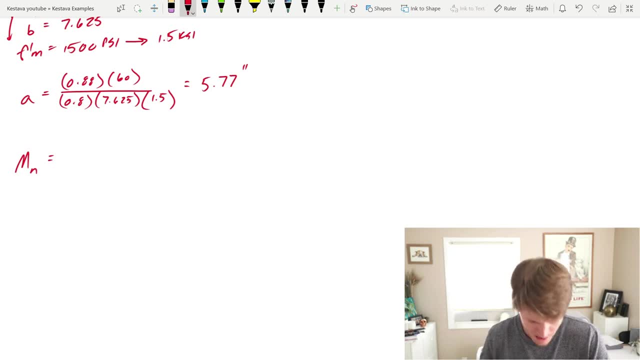 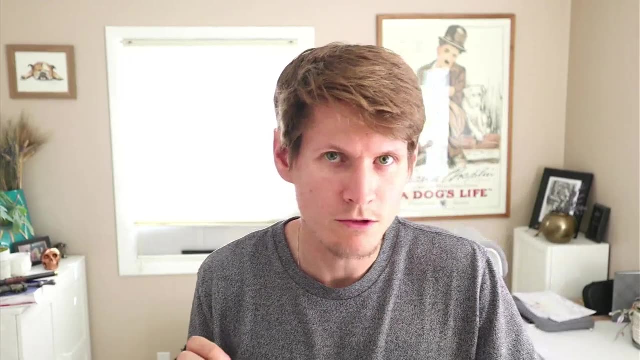 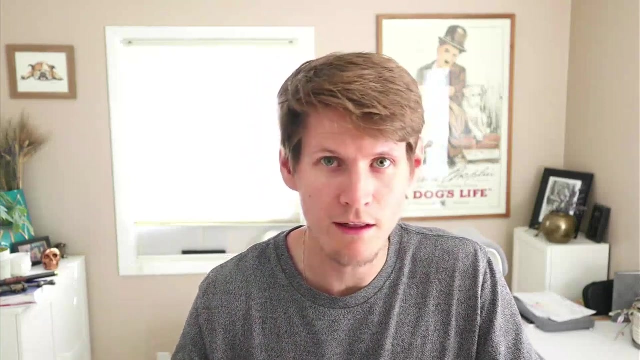 M. Let's try to find the moment capacity of our member. That's what the following equation looks identical to, concrete. And what's funny is you will notice when you do ASD design procedures, these equations vary slightly. Your properties of your steel and your masonry and all that kind of 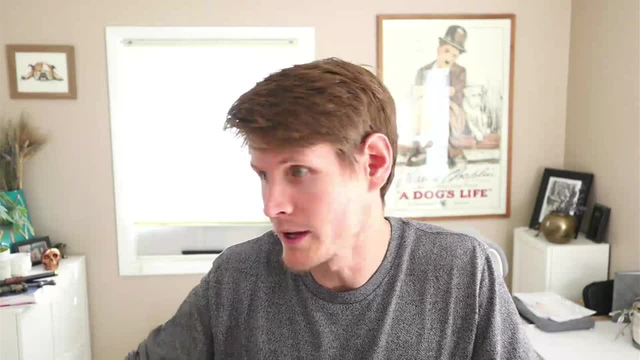 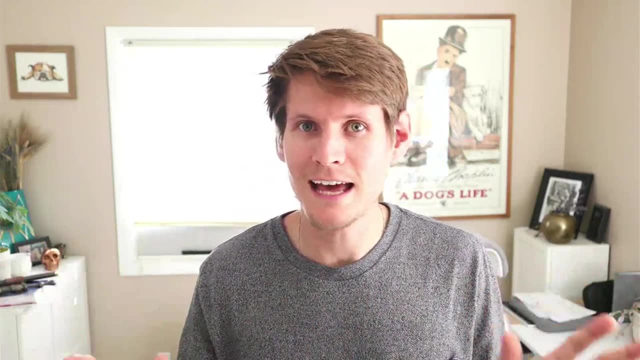 stuff that changes as well. There's factors applied to that, but your load combos are different as well. There are no load combos. and it's the same approach, but but different And from a numbers perspective. And it's the same approach, but different And from a numbers perspective. and 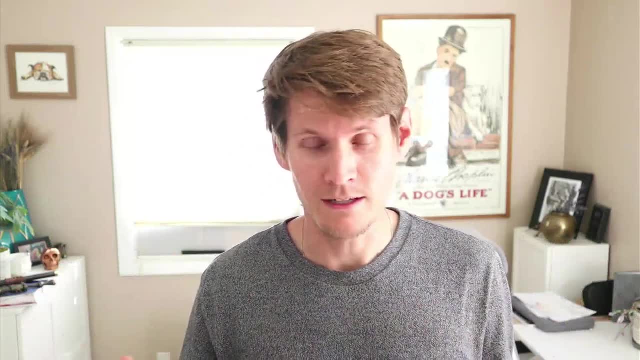 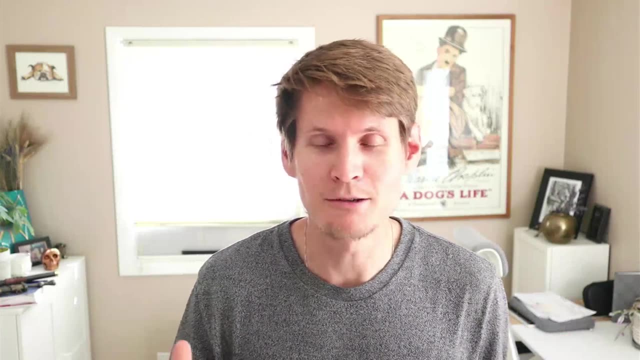 equations perspective, it can look incredibly different. So don't panic if you're skimming online and you're trying to find that question with the homework problem or whatever, and you see some procedure that is way, way, way different than you thought you were looking for. You just 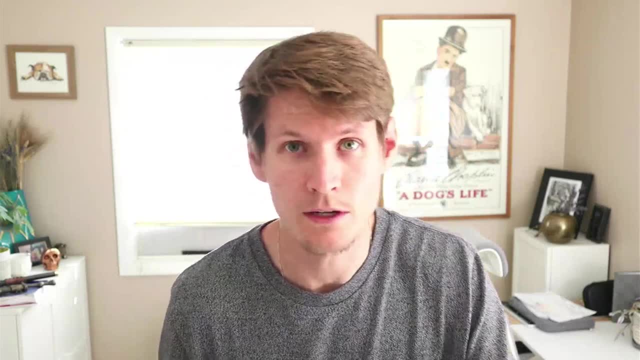 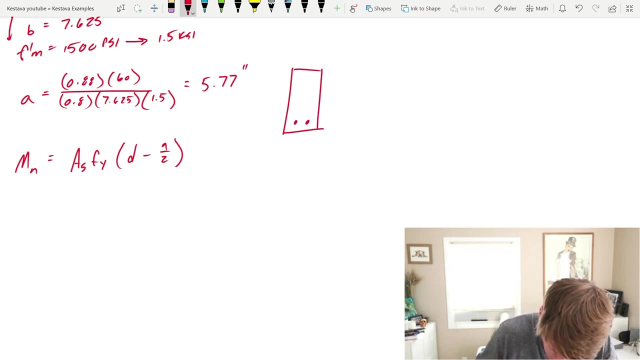 need to pay attention that there's two different procedures and they are different from one another. Let's keep going. D. this is the effective depth down to our flexural rebar, which was up above, but I'll just draw it here: Forty five inches. 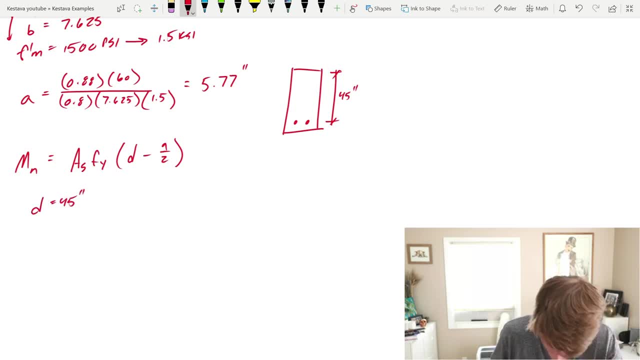 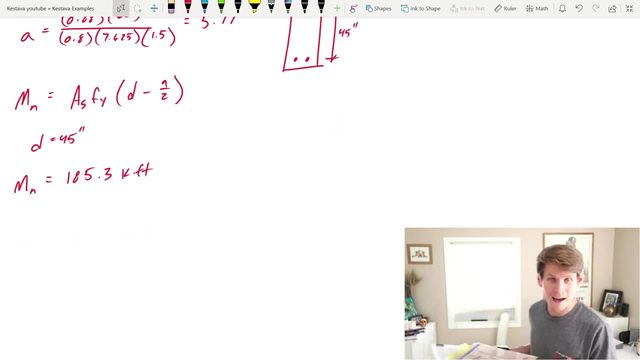 Full depth of 48 inches, So D that was easy. ASFY we have from above, A we solved, So let's plug all that in. MN equals 185.3 kip feet And unfortunately I don't have an electronic. 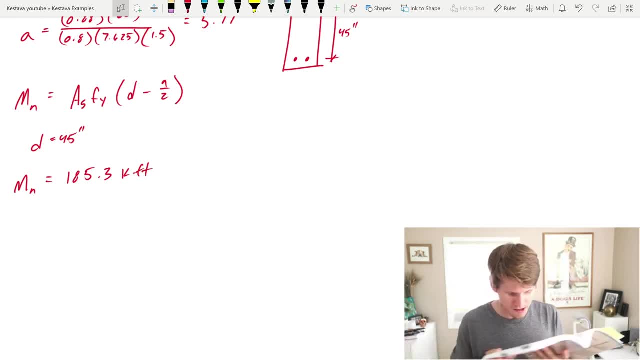 version of the TMS, but here it is right here. Next, you would need to find your fee for flexure, and that's in TMS. here I'll write it down. Well, it's 0.9 for flexure and that is TMS. 402 602 2016. 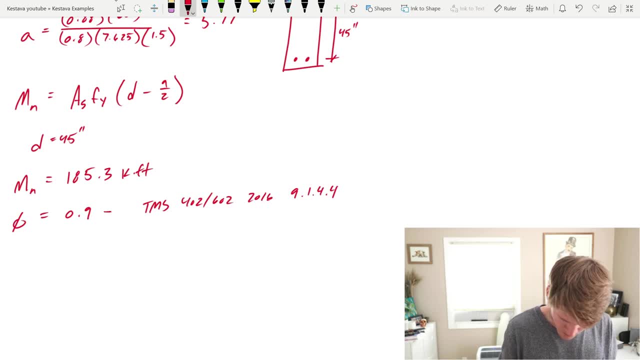 9.1.4.4.. That's where you get that sucker from. And chapter eight, I believe, is the allowable stress design procedures And then chapter nine is the strength design procedures And you don't have any fee factors in allowable stress design but you do in strength design. 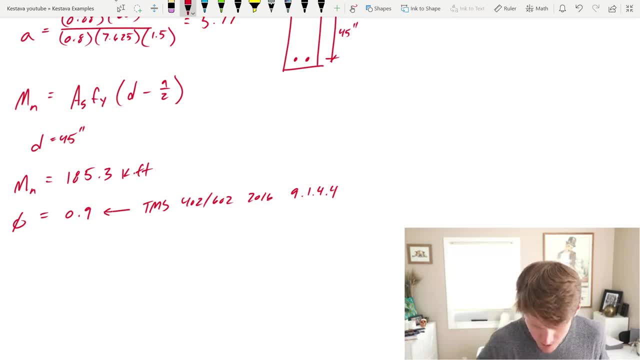 Again, that back and forth, that ping pong. But we've talked about it, so I'll get over myself and move on. You know what to do from here. Fee MN equals those two combined, which gets you 166.7 kip feet. Beautiful, All right. Well, we've determined the capacity of the masonry beam. 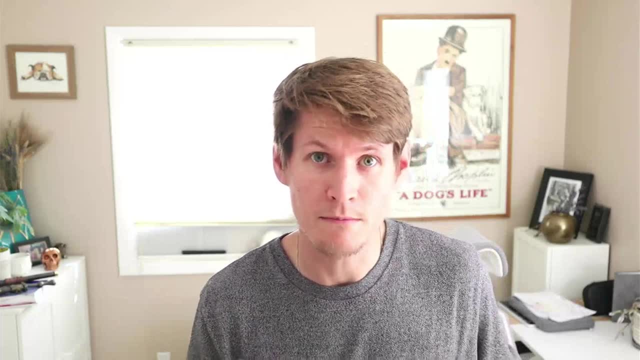 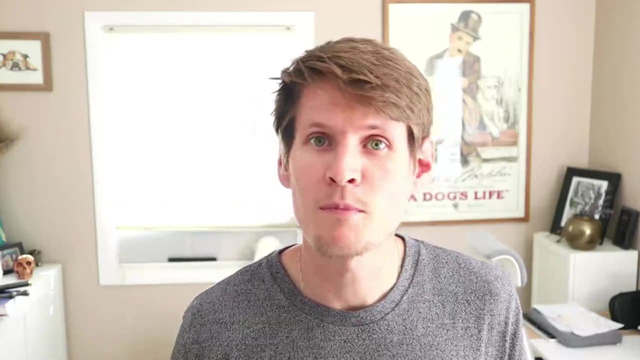 but now let's check for minimum steel reinforcement and maximum steel reinforcement. Make sure we're within code guidelines, because that's another huge thing. It's not just about strength, There's also all these other parameters that go along to make sure that we're designing. 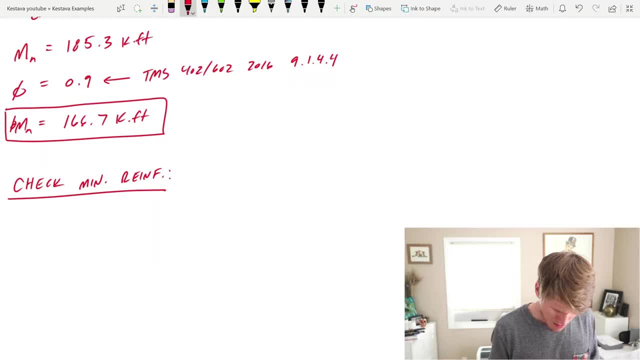 safe, efficient structures. And of course, I have the TMS out again, but this is per 9.3.4.. 0.2,, 0.2, 0.2.. All right, We freaking, get it MN, which we solved for. 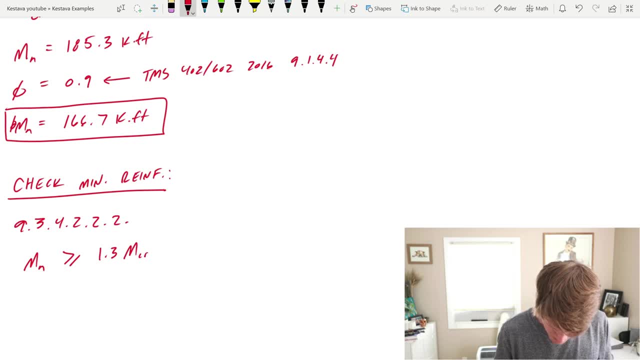 must be greater than or equal to 1.3 times MCR, MCR being the nominal cracking moment of the beam. And now you're like: what's MCR? Well, hang on a second Jeez, Louise. MCR is equal, very simple. 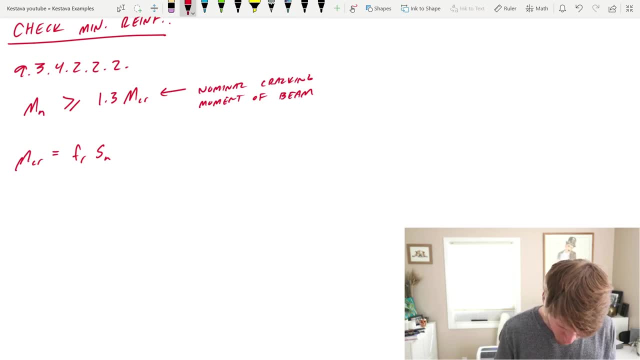 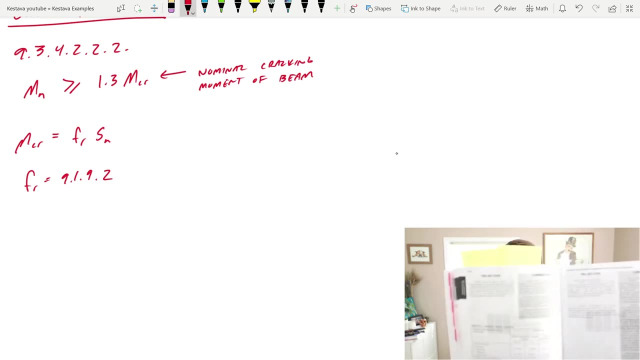 FRSN And FR is the modulus of rupture And FR can be found in 9.1.9.2. And it's simply a table that's given based on some parameters of your CMU number. We will say that we're using S-type mortar and the direction of flexural tensile stress is parallel. 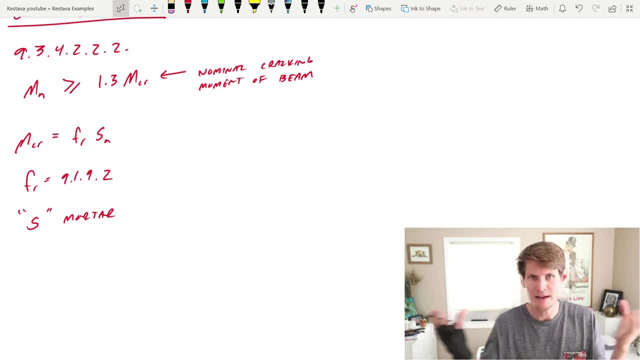 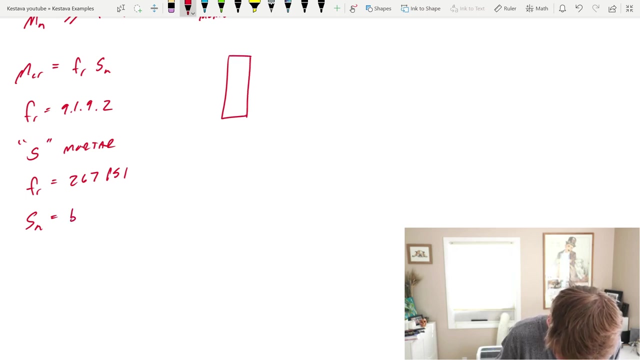 with the bed joints in running bond, because we have a beam and then our tensile reinforcement is parallel in that beam. F, prime, R or sorry, just FR, equal to 267 PSI S sub N- we all know we got a cross section is just equal to BH squared over six, which gets us 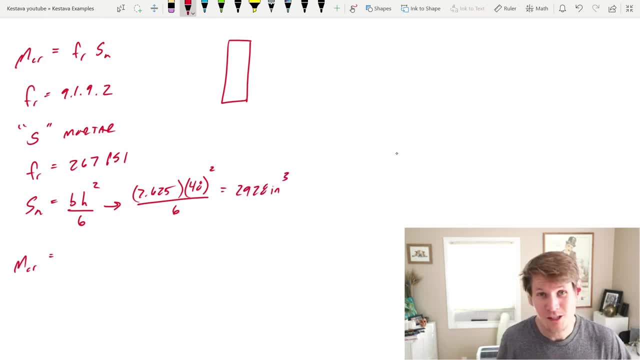 2,928 inches cubed MCR is equal to then 65.1 kip feet, And that's after you divide by a thousand, you divide by 12.. Make sure you keep all of your units consistent. It's very important throughout. 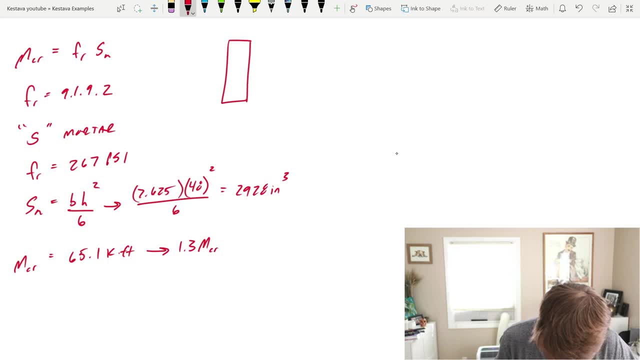 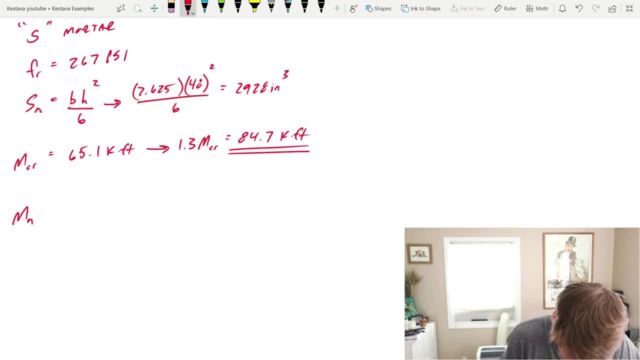 And now, if we take that and we get 1.3 MCR, that gets us 84.7 kip feet, And that's really the bread and butter, what we're looking for for this. check M sub N, not phi M sub N, just M sub N, which is equal to 185.3 kip feet. 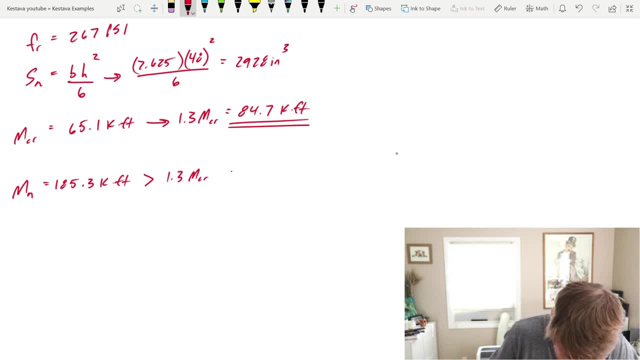 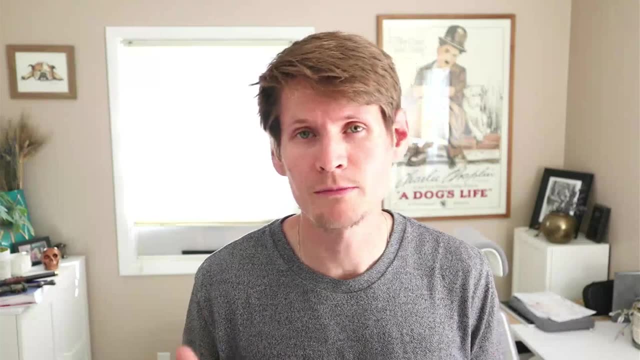 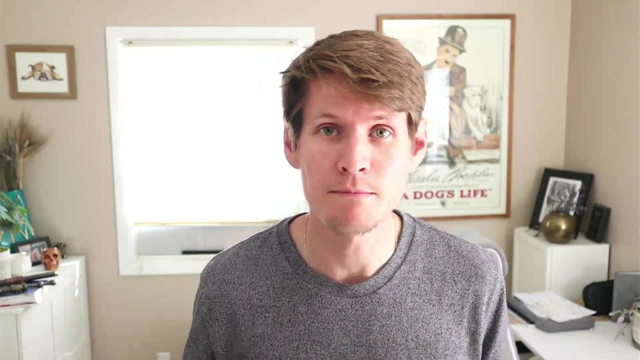 has to be greater than 1.3 MCR, which it definitely is. So we are okay, which means that our check is complete. for minimum reinforcement, We are okay, And this check, ultimately, is to make sure that we don't go away from brittle failure modes in the masonry member that we're designing. for lightly reinforced steel members. That's ultimately what this check boils down to, And in order to achieve this, the nominal flexural strength needs to be greater than 1.3 times the cracking moment strength, And that was just determined in laboratory testing through. 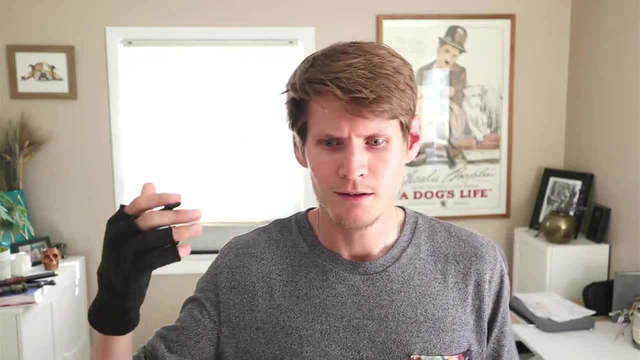 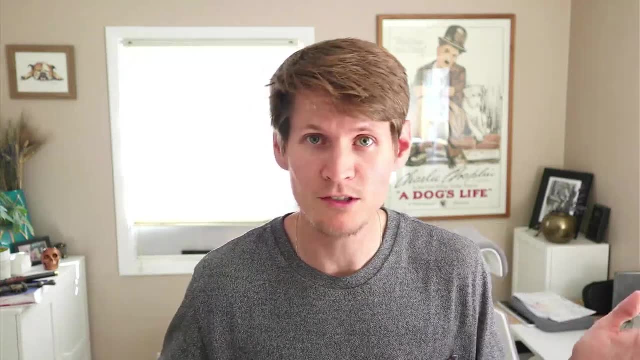 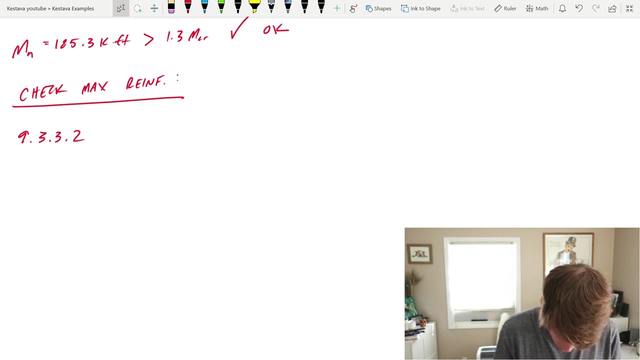 destructive. you know, tests over countless amounts of samples and studies to determine that that's what it took in order to bypass that failure mode. Simple as that. All right, let's check for maximum reinforcement. This is governed in the TMS in section 9.3.3.2.. 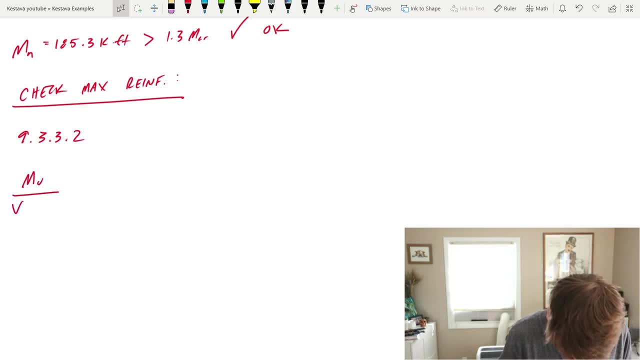 And, first off, what they want you to do is determine the following: MU over VD, times DV. And you need to make sure, or you just need to check and compare what this is, whether it's that, whether it's that to 1.0. And then you go from there and follow the steps to make sure that. 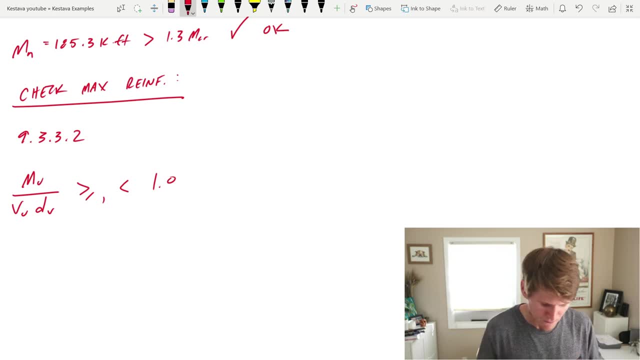 you're below these maximum reinforcement checks. But first off, we need to determine what this is. So MU is easy. That we already know is 86 kip feet VU. we would need to go back and you just need to run your- you know your loading on top of your simply supported beam to get your end. 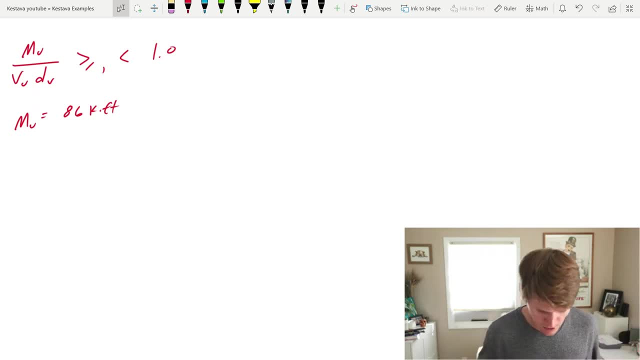 reactions, where your VU would be, where your ultimate shear demand would be. But we're not going to do that right now. But if you trust me enough, that gets you 34 kips, And that's factored, because this is, this is strength. design DV is the. 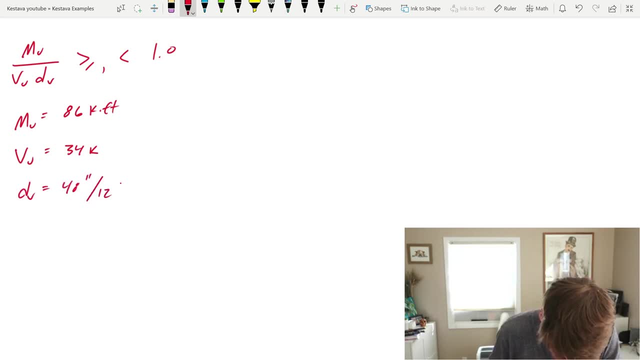 total depth of the member And we're going to keep this in feet, So we're going to make that four feet. We plug all this in MU over VU DV gets you 0.63, which is less than 1.0.. If you're greater, 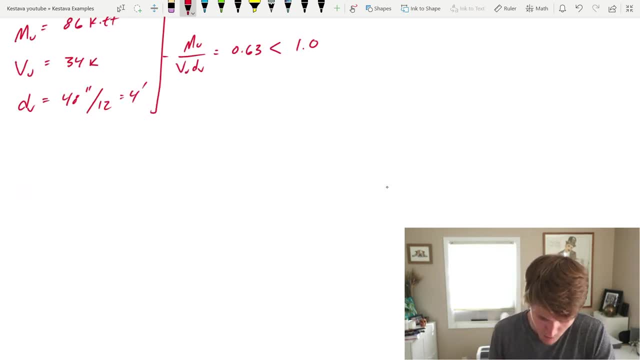 than 1.0, a lot more things start to happen. but if you're less than 1.0 per 9.3.3.2.4,- I know it sounds so dry- It's not the worst code in the world. I don't mind it that much. I haven't used. 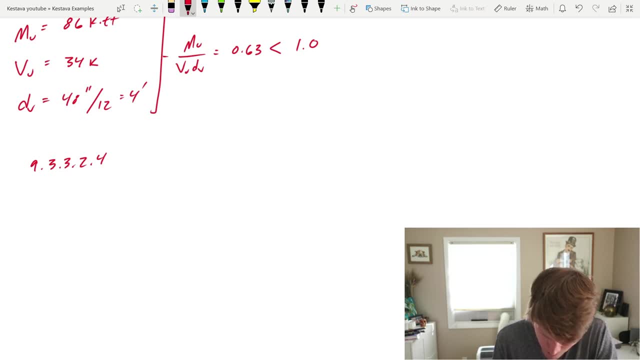 it a lot, but through studying it they did a pretty good job. I think they state that there's no upper limit on reinforcement as long as this value is below 1.0. So there's no additional check. We know that we are just good As long as your capacity of your member exceeds the demand on. 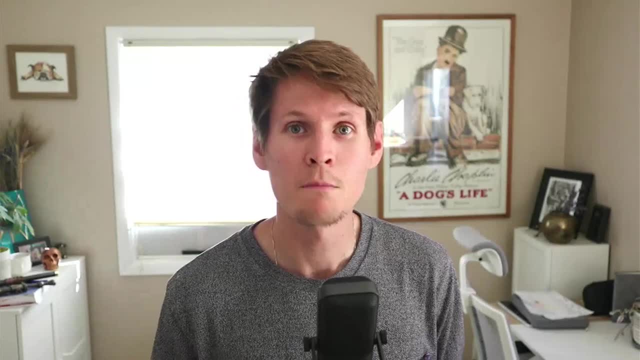 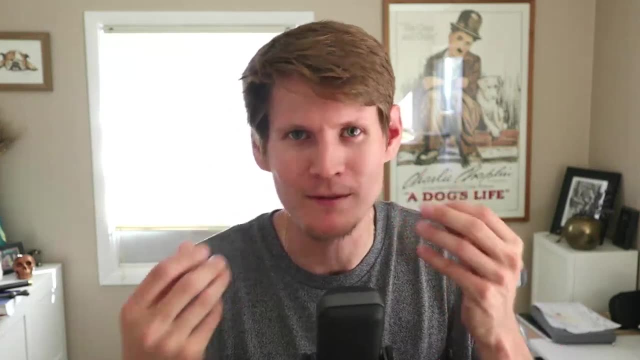 your member, And it's as simple as that. We are okay. Before you leave, If you did learn something new, I'd appreciate a like down below, but you don't have to. you know, it's just like those pity likes that I, you know, I just gobble up, But seriously, if you did learn something. 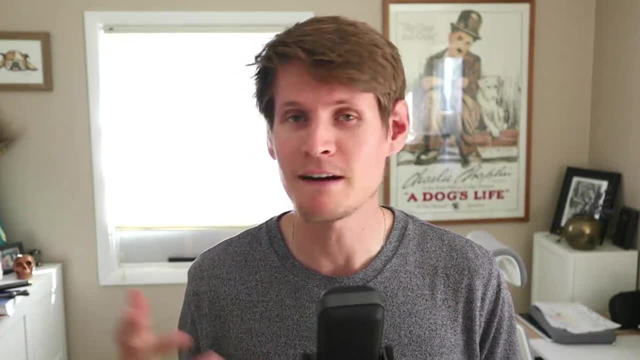 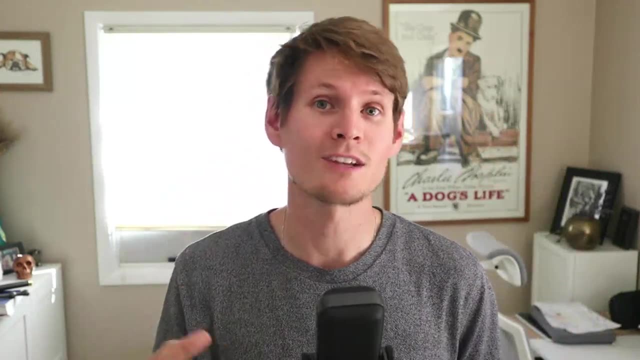 if you're feeling a little more confident about CMU, hit that like button. if I missed something, let me know seriously down below in the comments. I am studying this stuff right now for a test in October And I need all of your help to let me know that. Um, and if you're still here and you're